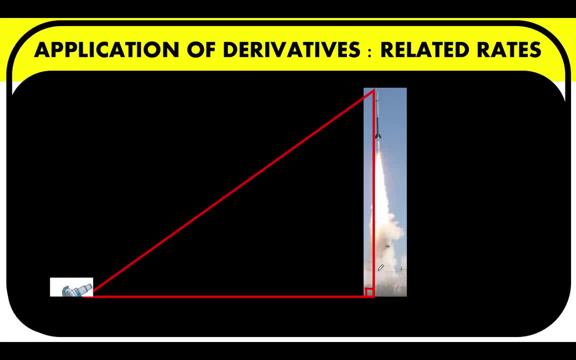 Okay, let's solve this problem together. You have a racket that's rising vertically- That means the angle here is 90 degrees- And you have this camera that is tracking the movement of the racket. The angle formed between the horizontal ground and the line upside to the tip of the racket is variable, denoted by. 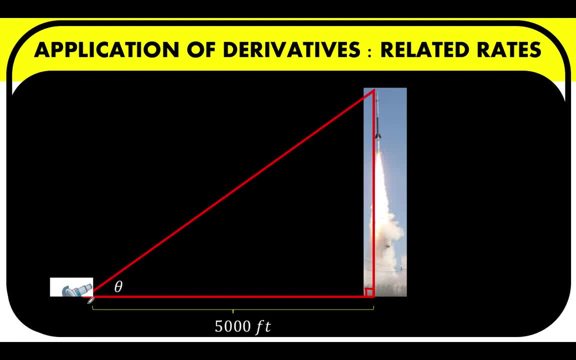 theta, And there is a fixed distance between the camera and this point where the racket is launched, and that distance is 5,000 feet. Let's call this variable as h, for the height and the hypotenuse as, let's say, 0.. 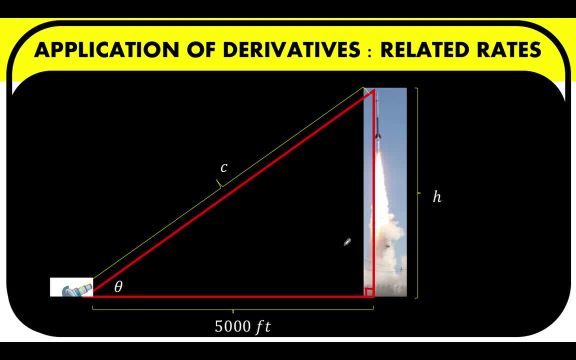 Now, based on our figure, we can now compute the ratio between the height and this horizontal distance and opposite over adjacent side with respect to the angle. theta is tangent. So we have tangent of the angle. theta equals the opposite side, h over the adjacent side: 5,000 feet. 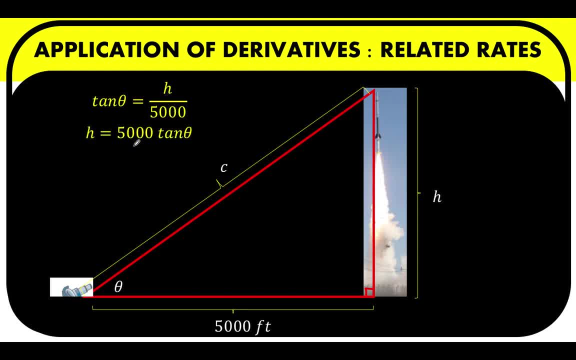 And then let's solve for h to arrive at. h equals 5,000 times tangent theta. We would like to know the rate of change of the height that is attained by the racket with respect to time, So we can now perform implicit differentiation for this equation. 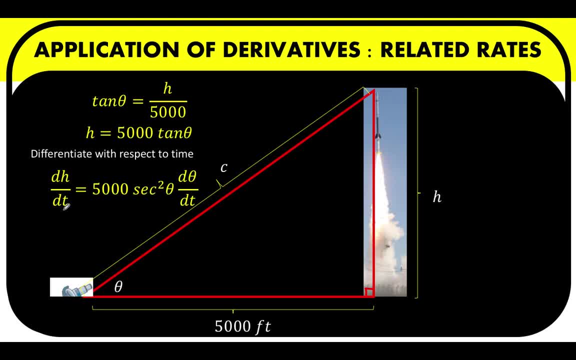 So, differentiating with respect to time, dh over dt is equal to this constant 5,000 times the derivative of tangent theta, which is equal to secant squared theta, d theta, because we are differentiating with respect to time. Now we need to find what is the value of second squared theta. It is given from: 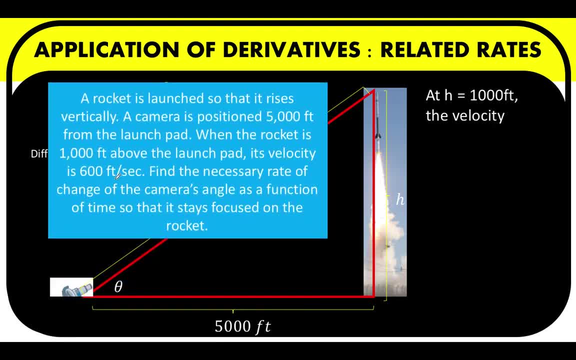 the problem that at h equals 1000 feet, the velocity is 600 feet per second. So we can now write dh over. dt is equal to 600 feet per second. That is the velocity of the rocket with respect to the time or the change in height with. 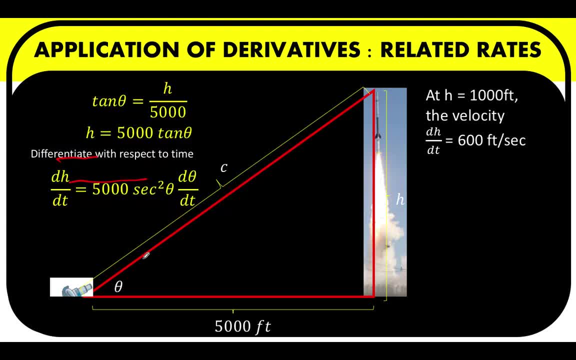 respect to the infinitesimal change in time. Now, since we have here a right triangle, we can now use the Pythagorean theorem in order to find the value of c. The hypotenuse is equal to the square root of the sum of the squares of the. 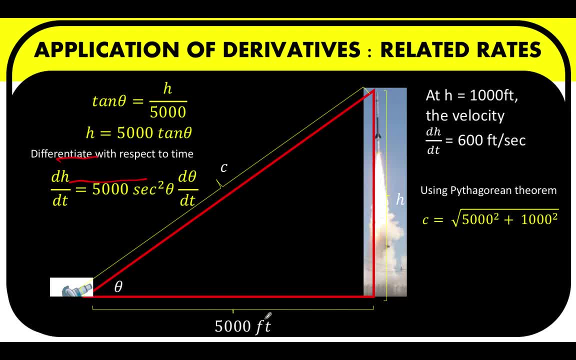 two legs Here. this distance is 5000 feet and the height is 1000 feet when the velocity is 600 feet per second. So whatever value for c that we'll compute here is the velocity of the rocket with respect to the infinitesimal change in. 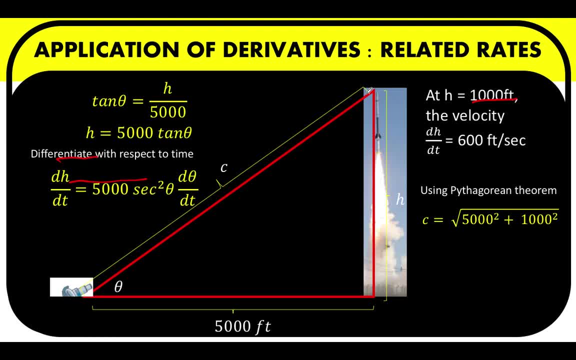 height. That is the length of this hypotenuse at that specific point, when the velocity of the rocket is 600 feet per second. So solving now for c 5000 squared plus 1000 squared equals 26 million, and getting the square root of: 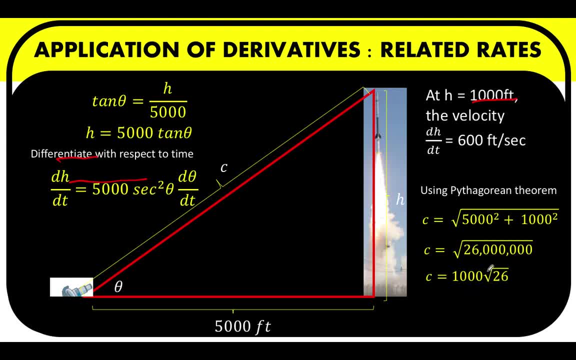 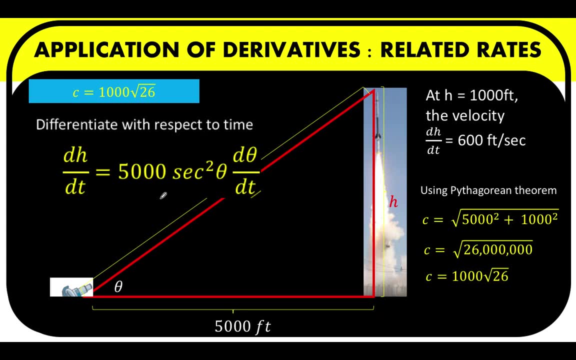 26 million, we arrive at 1000 square root of 26 feet. That is this distance c. Using now this value and remembering that we are solving for dh over dt, given by this equation that we arrived at previously, which is 5000 seconds squared theta d, theta over dt, we can now: 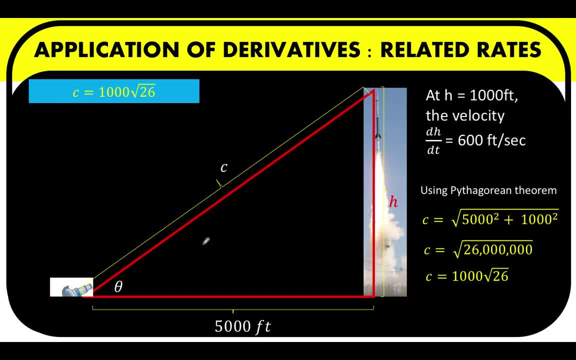 compute for this secant squared theta. First we need to recall what is secant theta. secant theta is the inverse of cosine theta. So if cosine is adjacent over the hypotenuse, the secant is the hypotenuse over the adjacent side. So here: 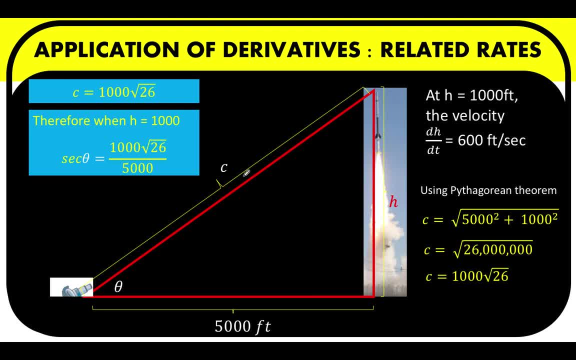 our secant of this angle theta is equal to this hypotenuse C, which we computed to be equal to 1000 squared of 26, when the velocity was 600 feet per second and the adjacent side is 5000 feet. We want the value of secant squared theta, so we 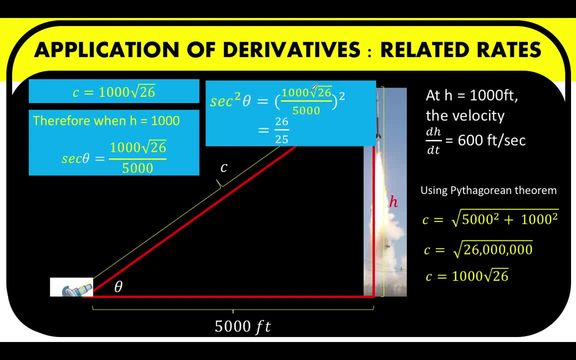 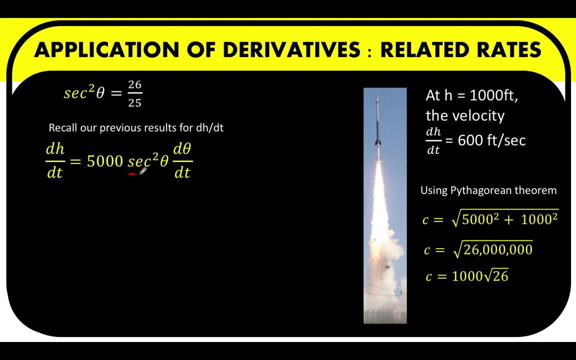 square both sides to arrive at secant squared theta equals 26 over 25.. This is now the value that we need to substitute in our preliminary results. So, using now this value for secant squared theta, substituting that value to this secant squared theta, when dh over dt or the velocity equals 600 feet per second, we 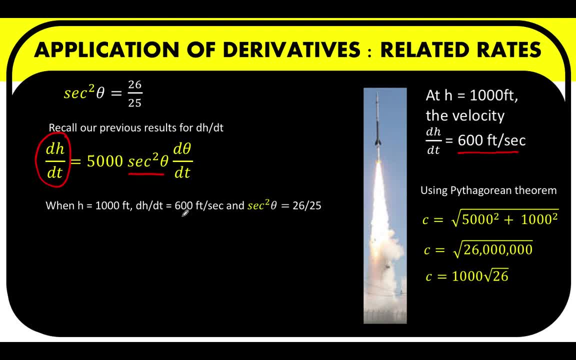 can now replace this dh over dt by 600 feet per second. We can now replace the secant squared theta by 26 over 25, and so we arrive at this result: you Now solving for d theta over dt. we arrive at a value of 3 over 26 radian per.